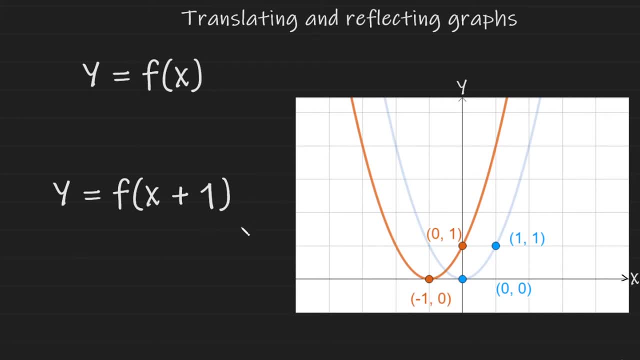 can conclude from this that translations to the inside of the function, so inside this bracket, work in the opposite way. Okay, time for our first reflection. I'm going to make the outside of the function, so outside of the brackets, negative, and that looks like this: This now changes the. 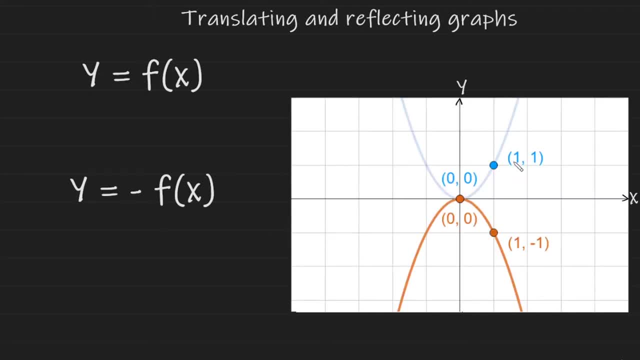 graph to look like this: If we look at the coordinates, the y values that were positive are now negative. However, this zero remains the same as zero doesn't really have a positive or a negative sign. We can conclude that applying a negative to the outside of the function. 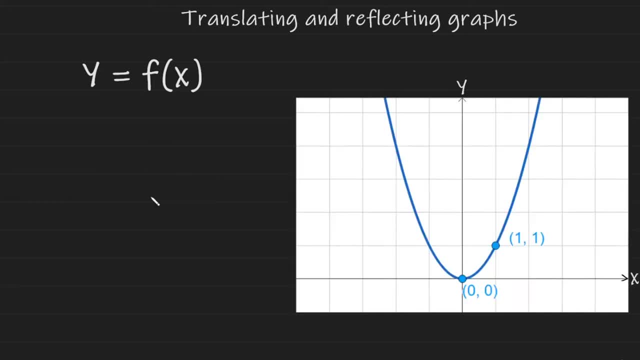 will reflect the graph across the x-axis. For our second reflection, I'm going to make the inside of the function, so inside of the bracket, negative and this is what it looks like. Doing this changes the graph to look like the following: If we look at the coordinates, the x values that were positive. 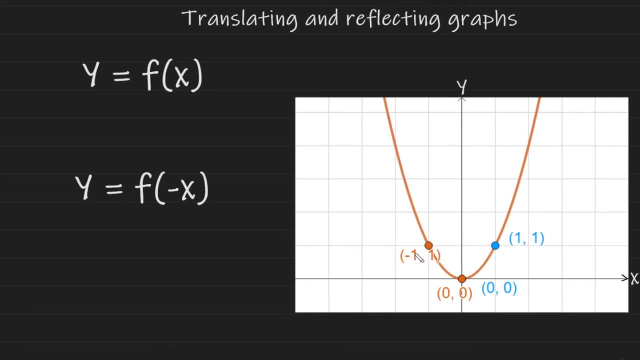 are now negative, So this one here now becomes a negative one. We can conclude that applying a negative to the inside of the function, so the inside of the bracket, which is also the same as a positive, as applying a negative to all of the x values, will reflect the graph in the y-axis, Because this 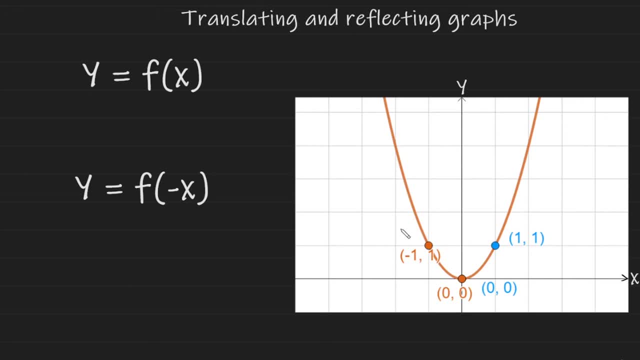 quadratic graph is symmetrical. the reflection looks the same as the original graph. Think about it. Look at the original again. If I reflect or flip it around the y-axis, it would still look the same. Okay, now let's use all of this knowledge and understanding to answer some typical questions. 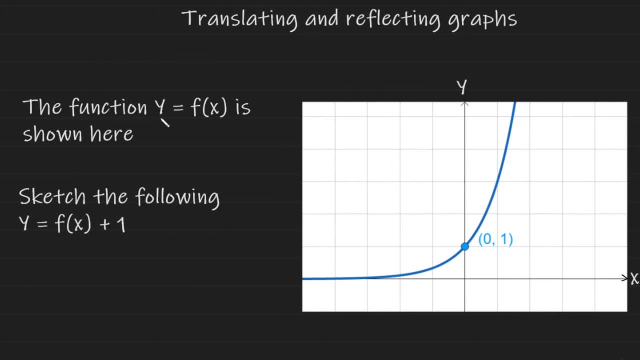 that you may get In this question. they tell us the function y equals f of x is shown here. This is an exponential function. They ask us to sketch the following: y is equal to f of x plus one. So this is on the outside of the 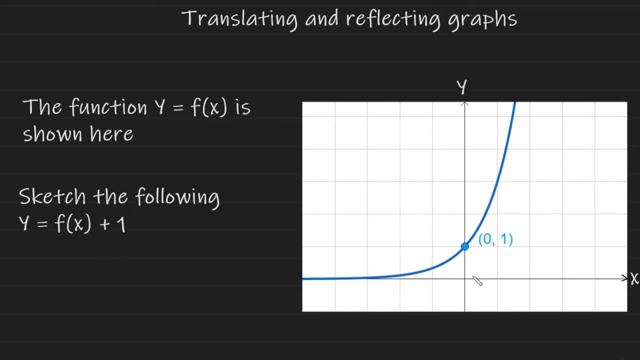 brackets. Therefore, it should translate the entire graph up by one. So this point here will no longer be zero and one. It should be zero and two. Also, this part of the graph which seems to be leveling off on the x-axis, but never actually touching it, should also move up by one. So therefore, the leveling off. 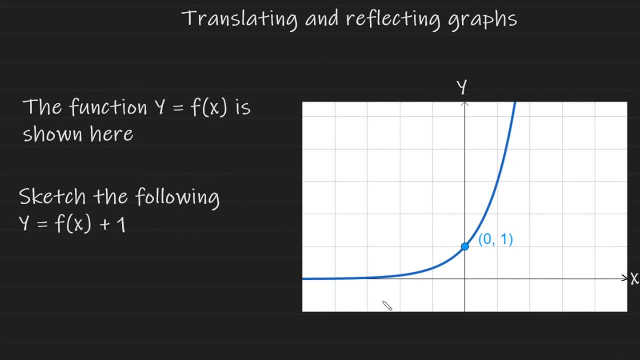 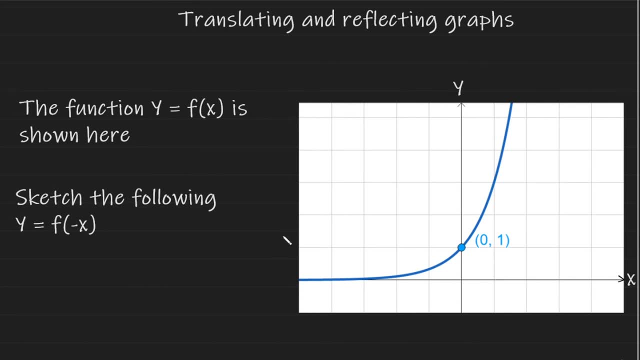 should be taking place here. Sketching this graph looks like this. As you can see from the previous explanations, the graph changes in the way that we'd expect. Okay, now for this question. the exact same function as before and the graph, But now we are being asked to sketch the following: There is a negative on the inside.